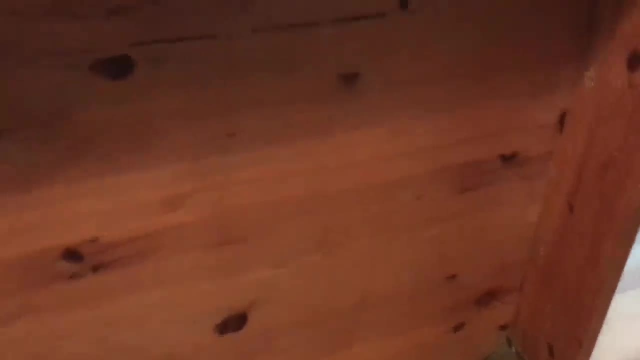 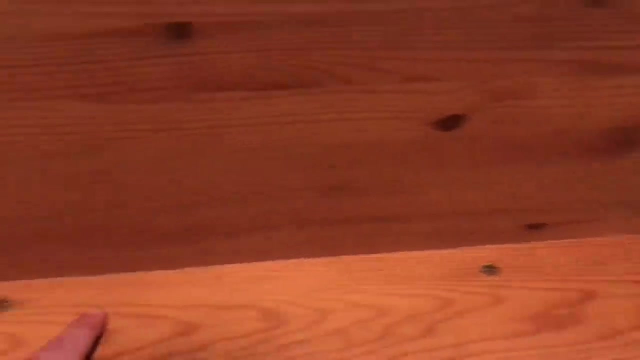 Now, this is what the underside of the table looks like, and the chances are it will look very much like one in your house. The table top itself is actually held on by a number of wood screws that are just put in at a diagonal to sort of hold it down. 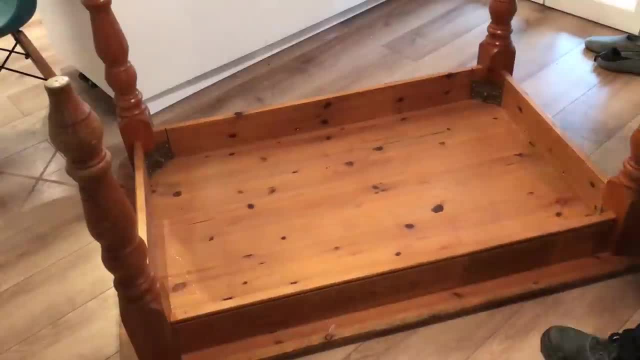 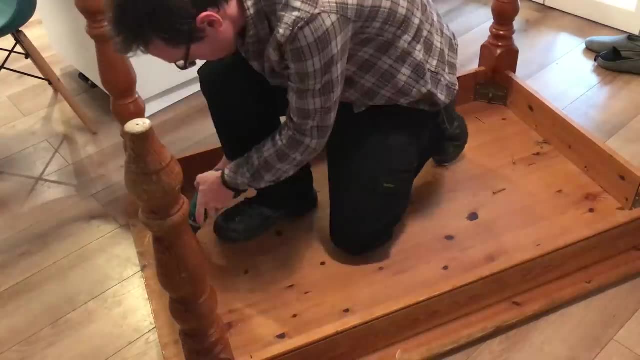 And in the corners are some brackets to hold the legs on. Now, taking the table top off is just as simple as using a power screwdriver or a drill to take these diagonal screws out. Once you've got all those out- and it might take a little bit to find them, as some of them are hidden away- you can just pop this side assembly off and remove the table top. 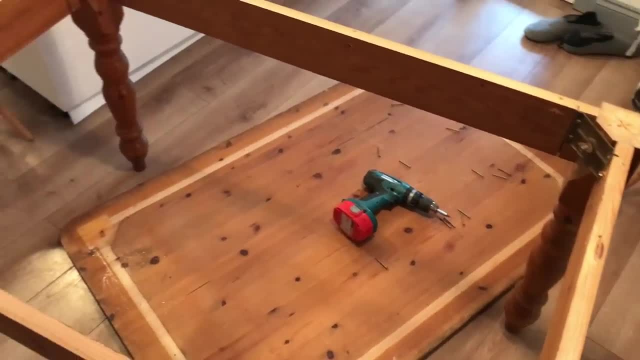 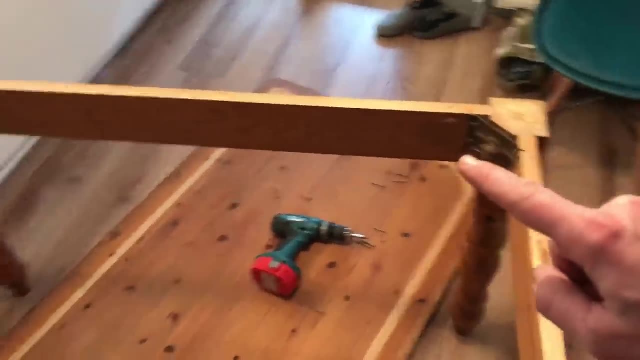 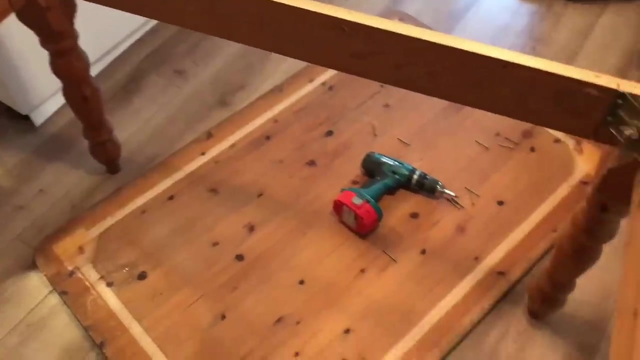 So, with those screws out, the table top comes off, and this is going to allow me to batten round using maybe some 2x1 timbers, whatever I've got lurking around upstairs to the side of the frame, And I'm just going to use some little self-tapping wood screws, much similar to the ones that held down the table top in the first place. 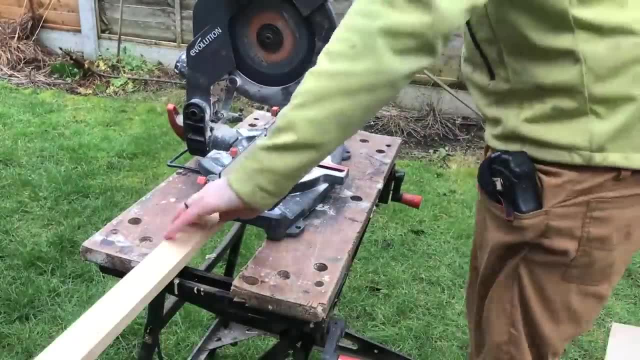 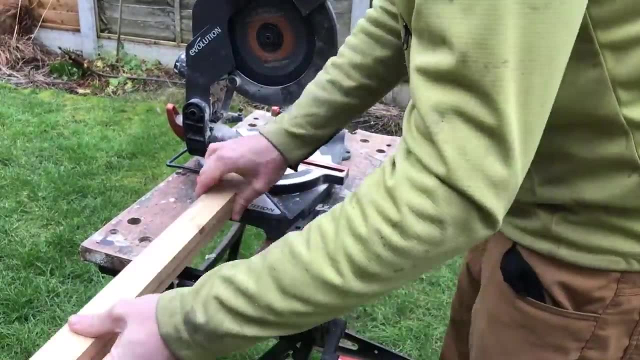 So these are the battens. It's 19x38mm kiln-dried, sawn timber. Probably a good idea to get kiln-dried so it doesn't warp and split when you get it in the house. But I've cut it using a cross-cut saw. You can just as easily use a tenon saw or any other kind of woodworking saw. 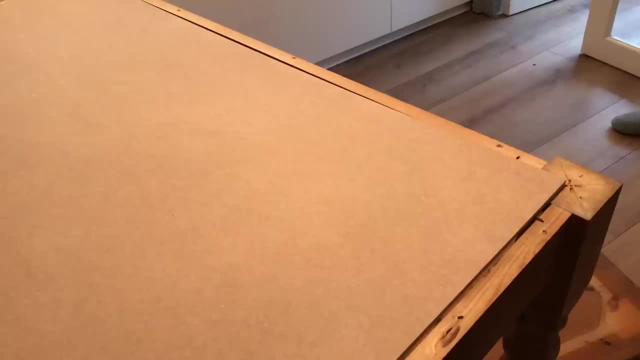 And you don't have to be that accurate, I've just measured them roughly to the size. So this little piece of MDF is going to form the gaming surface and this is going to sit below the level of the table top to create a little cavity here. 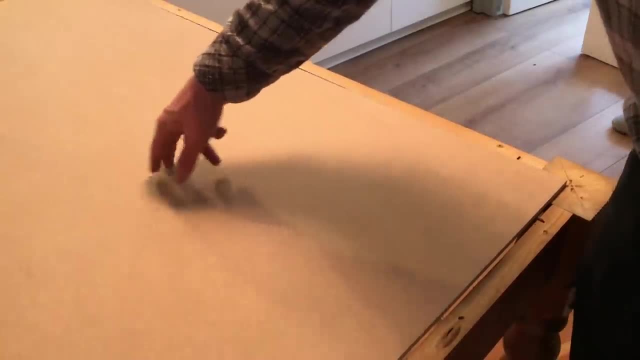 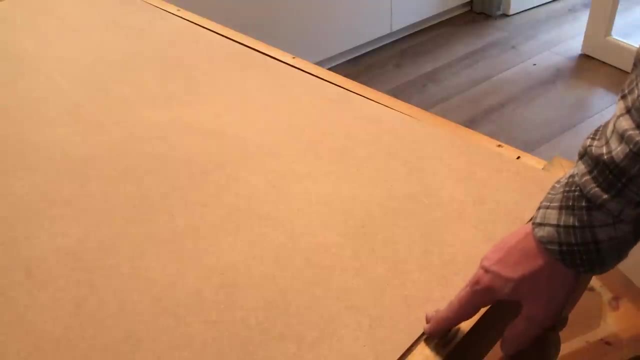 It's only 9mm MDF and it is a little bit wobbly, but I'm hoping that the battening around it is going to really firm it up Now. the reason why I've used 9mm MDF is just basically because I'm a cheapskate. 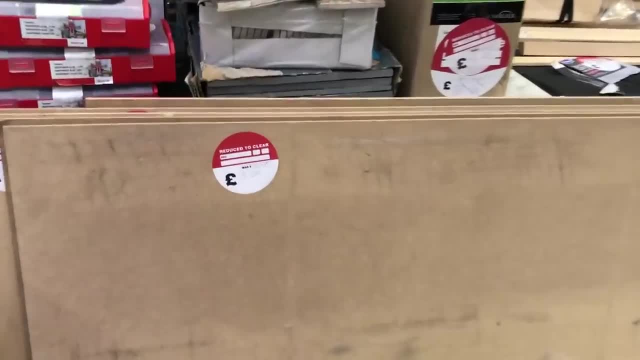 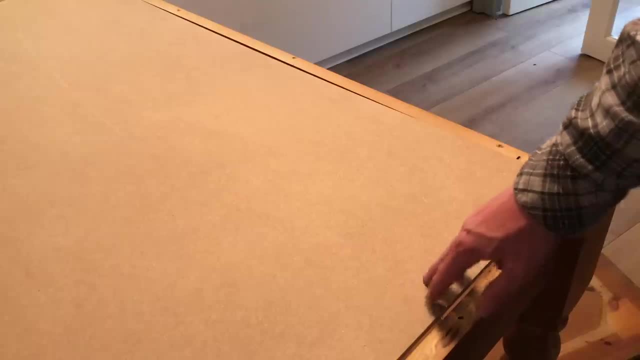 Wix, the local UK DIY superstore, has these sheets in its stores and they use them as a packing material to separate layers of laminate flooring. So they actually sell these and give the money to charity. So I've got this entire sheet for three whole English pounds. 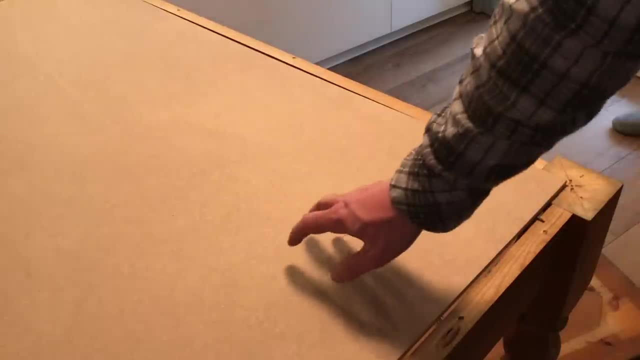 What's that About five US dollars? So I've basically gone with the cheap option, with the idea that I can beef it up if required. So while I was all set up in the garden, I got the MDF sheet cut to size. 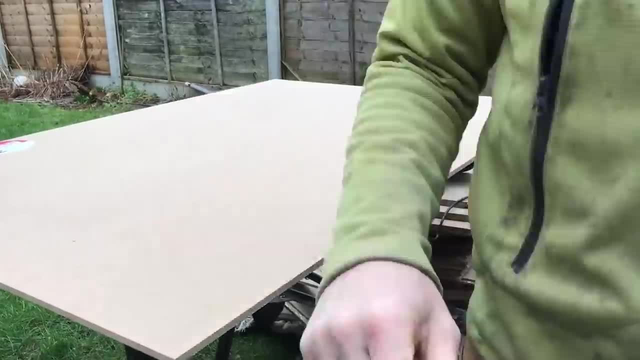 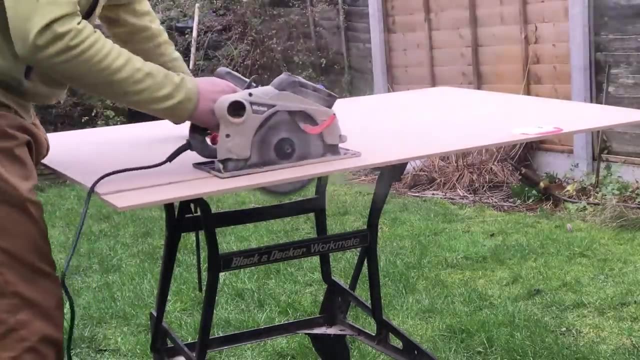 And it's a good idea to do it outside anyway. MDF dust is really quite nasty. You should really wear a dust mask if at all possible. So I've just used a panel saw just to cut along the length. You can see how windy it was on the day. 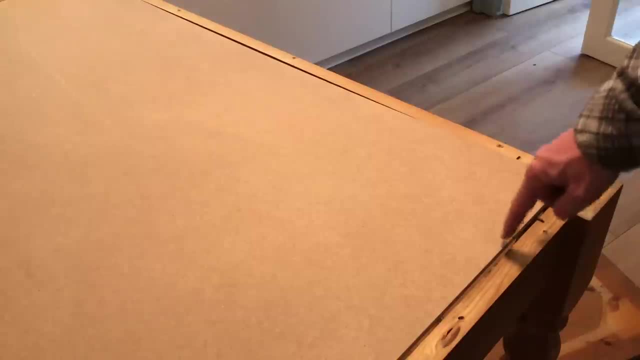 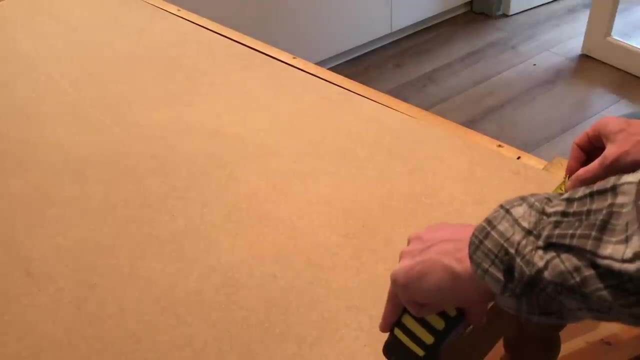 Now, as you saw before, across the corners are some braces that hold the legs in place, with these side elements here. So I'm just going to make a little measurement across and it looks like about 100mm, Actually a bit less. 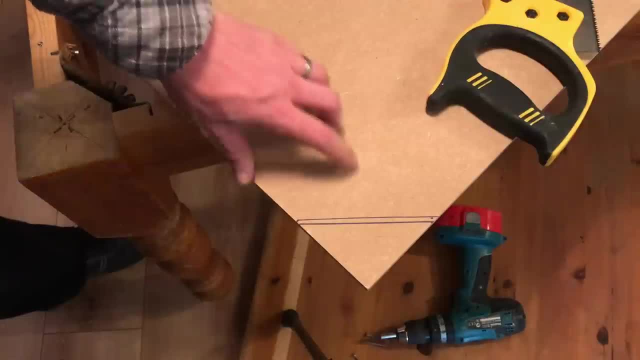 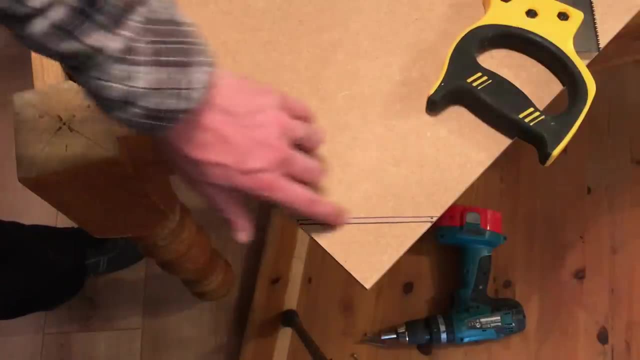 Let's have a look. I've done a bit of a think. The whole table seems to be imperial Feet in inches, So I re-measured this: Instead of being 80mm, being 3 inches, 45 degree that I'm going to cut off to create that relief for the corners. 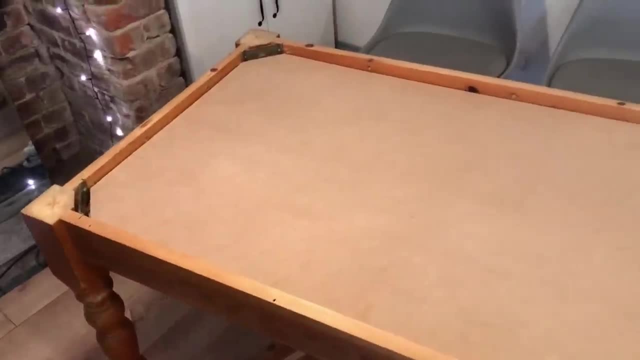 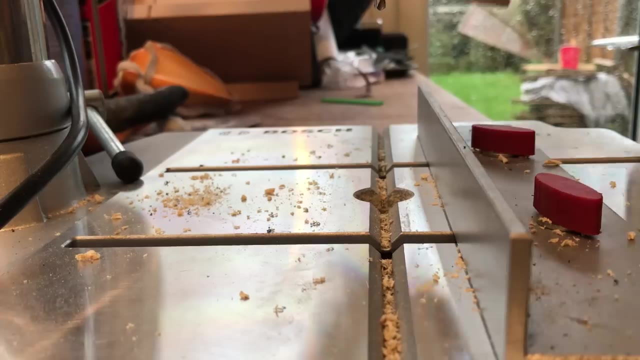 Okay, with the corners cut out. it just sits on top of those wing nuts in the corner. It's actually going to sit much lower down to create a greater depth so I can leave board game components out. So I pre-cut before. 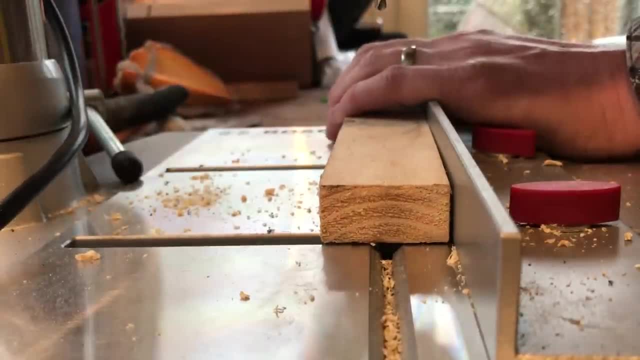 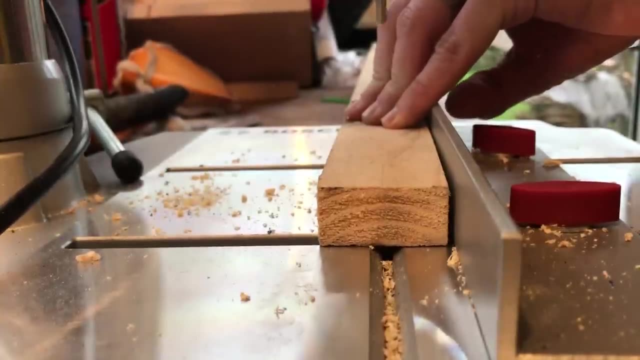 I'm just drilling three pilot holes. I'm drilling one at either end and I've just normally chosen one inch from the end And I'm going to drill one in the middle, one at the other end. That's just going to allow the wood screws to locate and I'll be able to clamp it up. 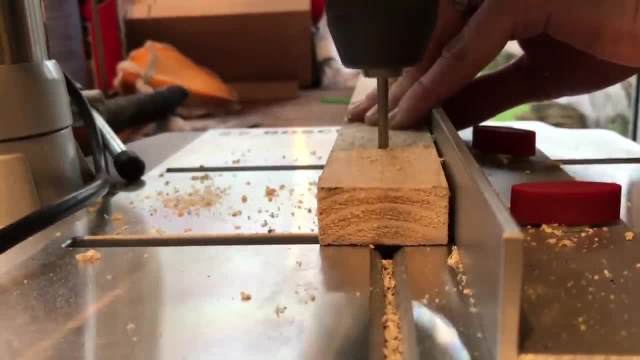 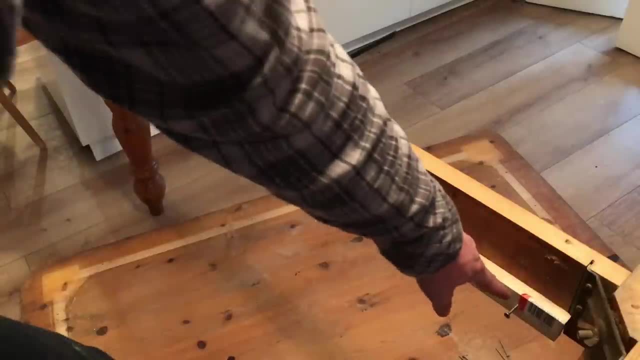 So hopefully I shouldn't have to do any complicated measuring. It's all just going to be done by eye, which makes this a really quick project. So with the battens cut to length, I've pre-drilled a clearance hole in three positions on the side. 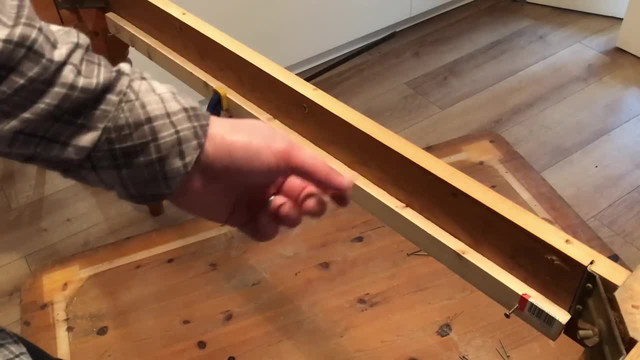 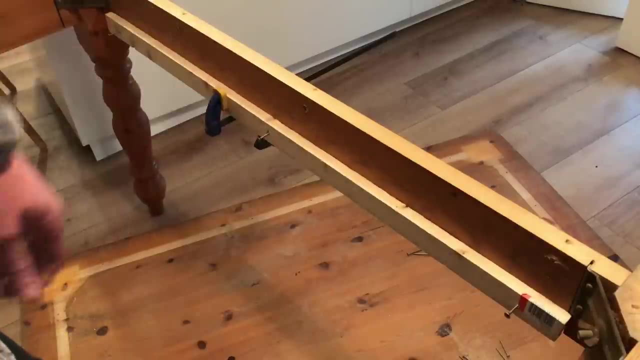 I guess I should really pilot this, but I've got some self-drilling self-tappers, So they're just going to go straight in there, and I've used a quick clamp Just clamp that up to hold it all in place. So let's get this first batten secured. 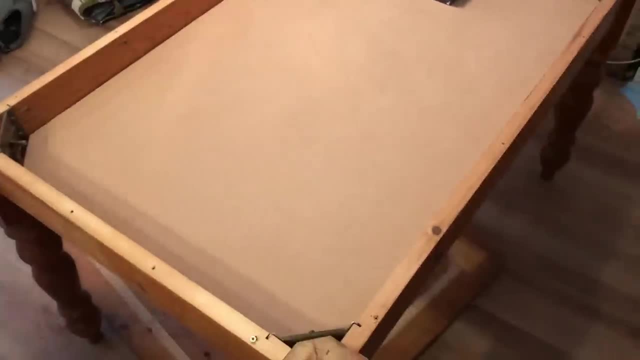 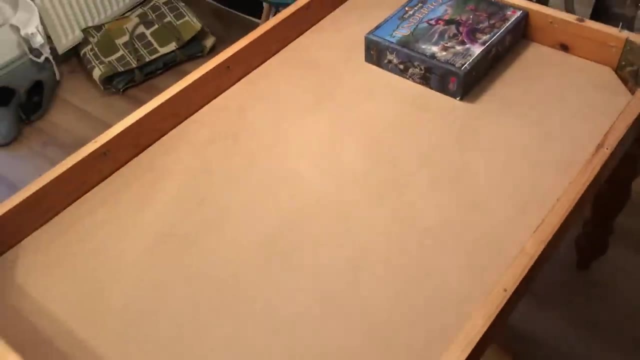 So we have the first fix of the sub-table, as I'm going to call it. It's only 9mm MDF, for the reasons I've discussed before, just because it's super cheap, But it's actually remarkable. It's remarkably stable and it's not even screwed down yet. 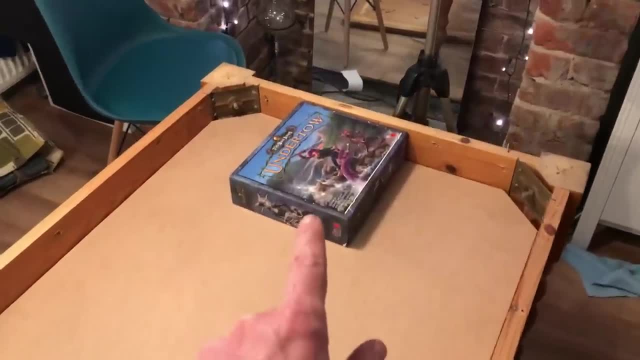 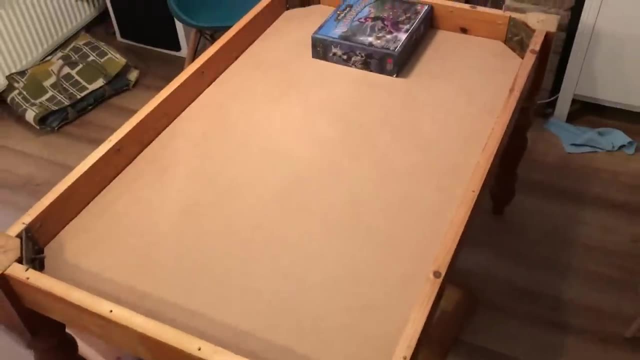 And just to show you, that's the Too Many Bones under-tow box, which just about fits under the table top. So the next bit is the exciting bit. I'm going to put the headliner felt and the gaming felt on and see how that goes. 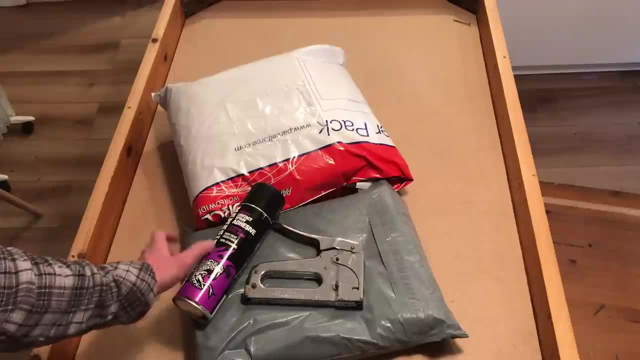 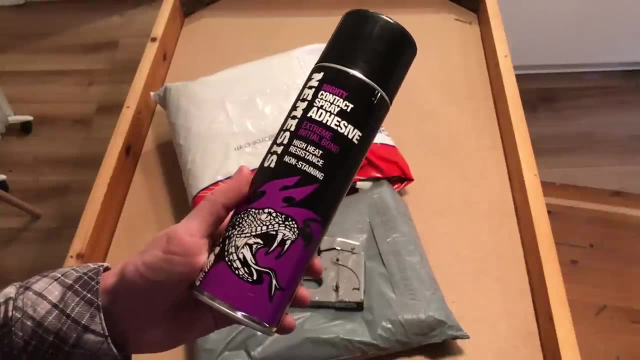 Okay, so not only am I not a carpenter, I'm not an upholsterer, So we're going to see how this goes. I've had a bit of research. I'm trying the products I think I need. So this is some contact spray. 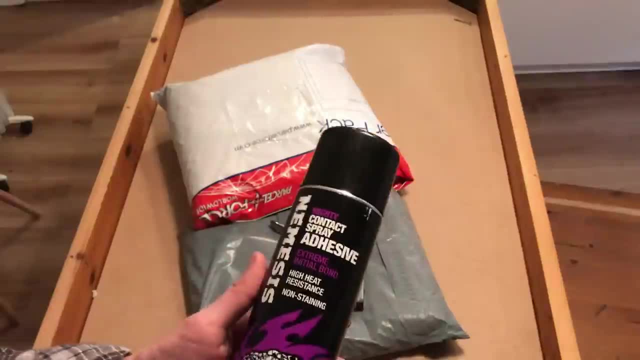 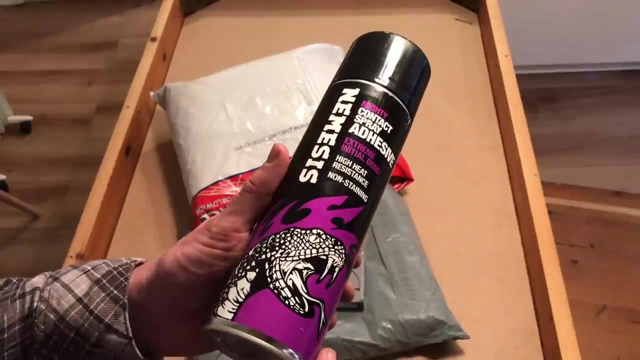 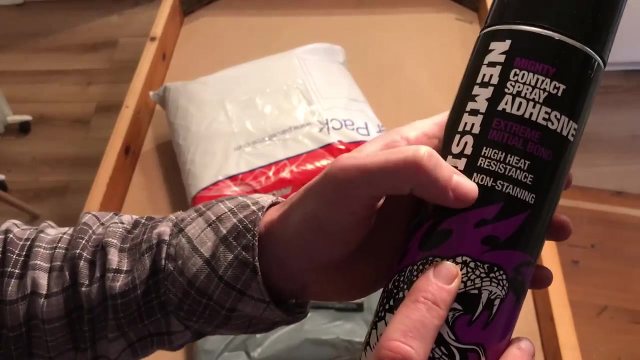 In my first video, where I made a little laptop gaming tray up here, I used some 3M contact adhesive spray. It wasn't great, to be honest. So this is the Heavy Duty Brother Nemesis contact spray adhesive- Critically non-staining as well. 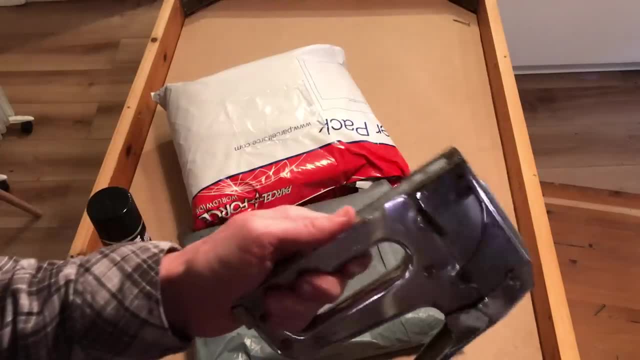 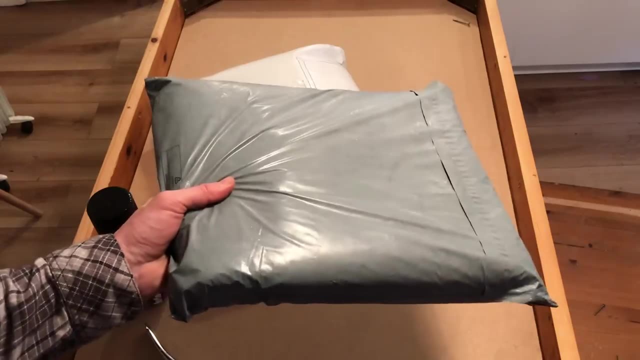 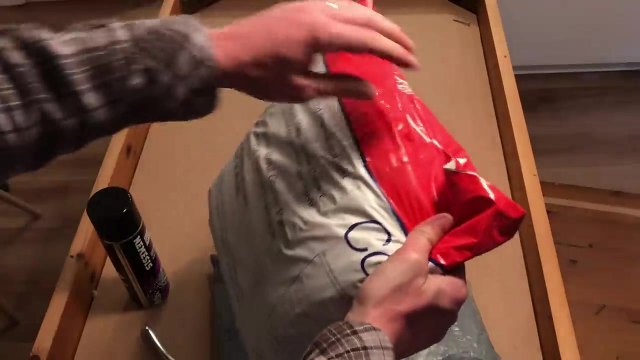 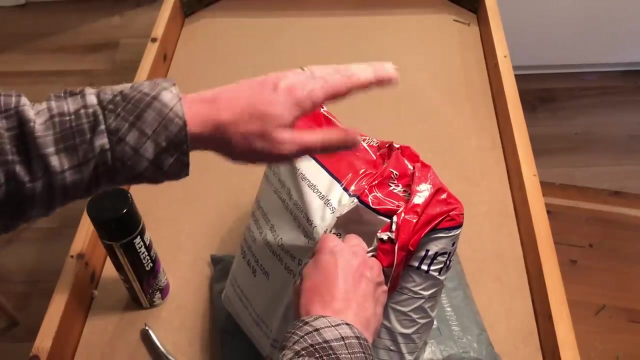 So it should be fabric safe. Get a bit of tension, I think will require a staple gun, And in these two packages are the fabrics of choice. So package one is what they call headliner fabric. Now, this is the fabric that goes on the ceiling of a car, as it were. 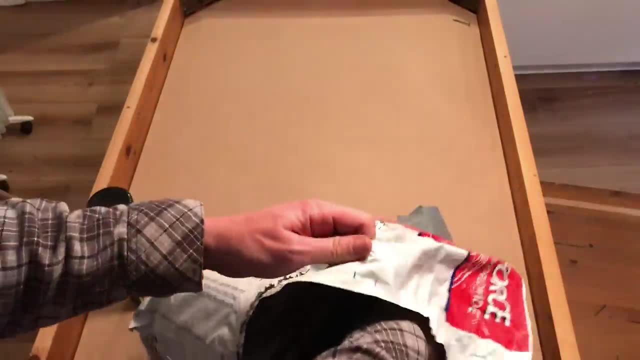 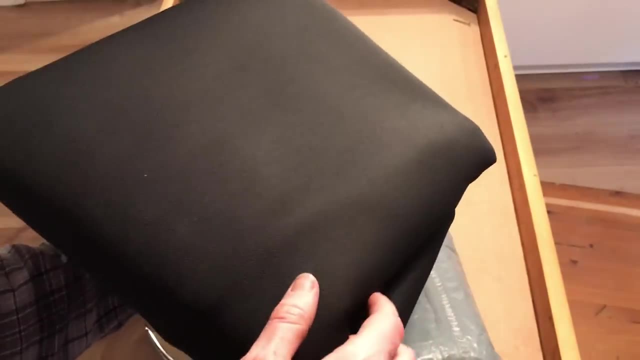 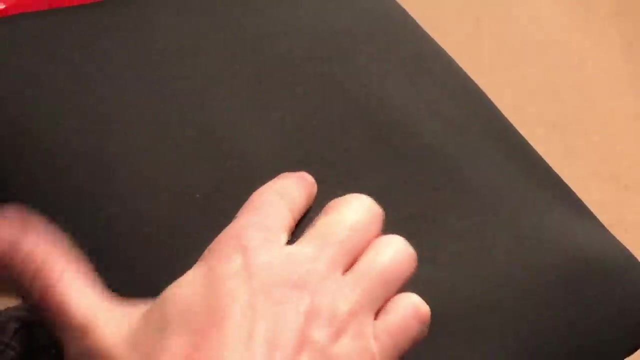 So let's have a look inside. Not relatively clean hands, Hmm. So that in itself is almost a nice gaming surface. See if I can just zoom in a touch. It's got a little bit of sponge to it and that's what gives the soft dice roll. you get on. 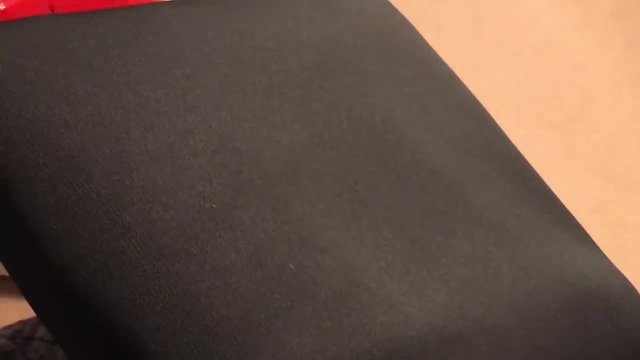 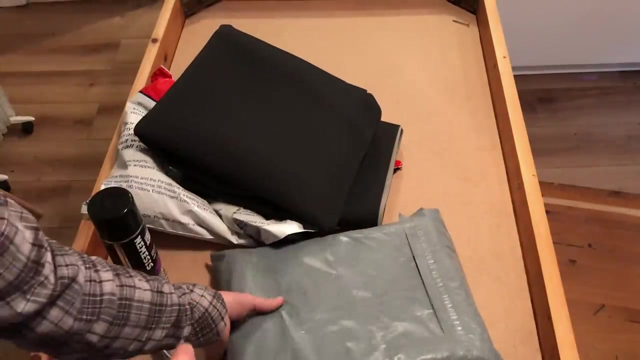 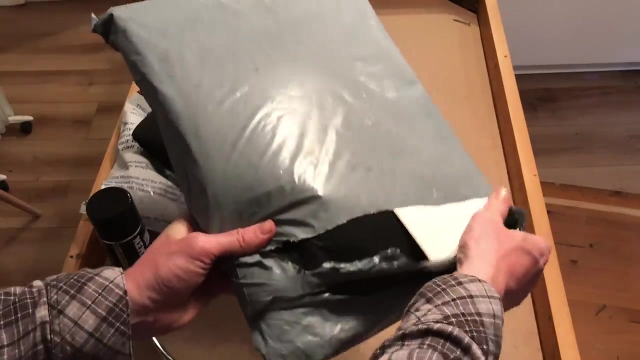 Nice casino style tables. Now I sort of struggled a little bit with the topper of choice. I went with a black felt. I think speed cloth might have been my preferred style, but I just couldn't find it in just a plain material. 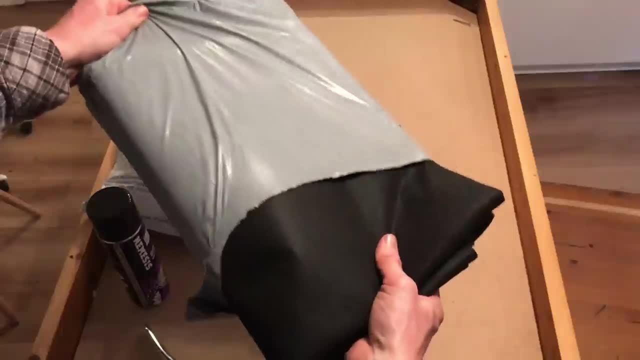 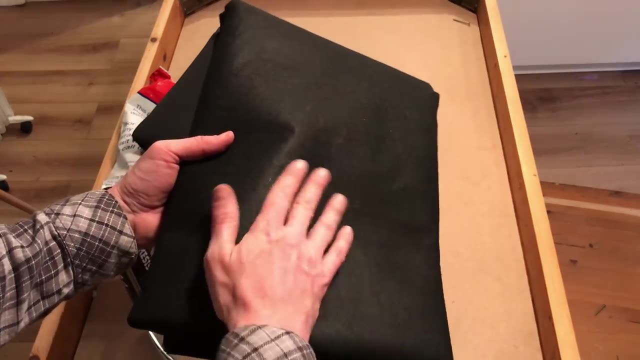 They all had the playing card suits that were embroidered into it, which I didn't want for my table, So I've gone for a standard black felt, And the thickness of this, along with the headliner felt, should give a really nice sort of premium feel. 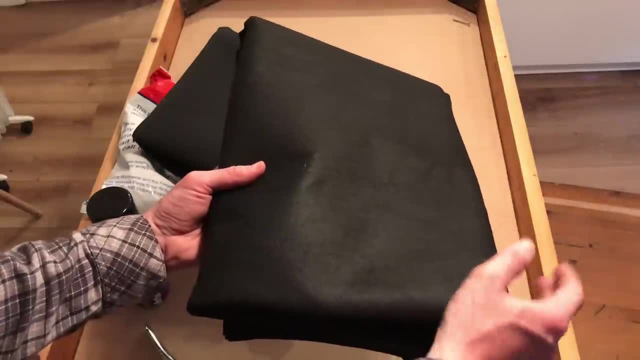 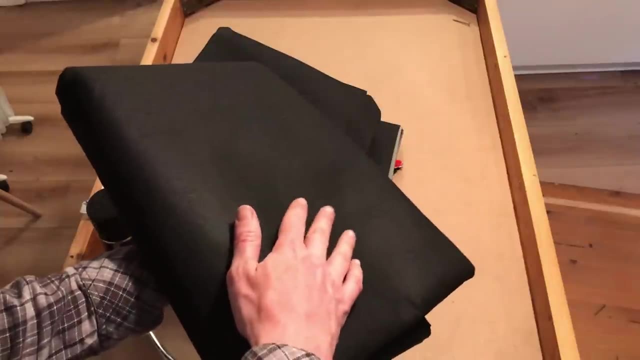 I tried the felt on its own on the lap gaming tray. It was fine. It's certainly a lot nicer than just playing on a table, But I don't think it's going to give that premium quality feel that a pair of these fabrics will give. 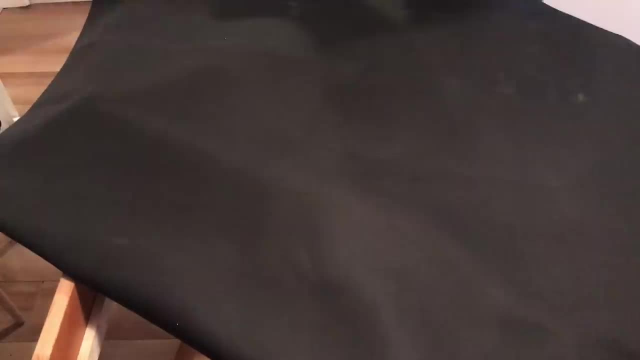 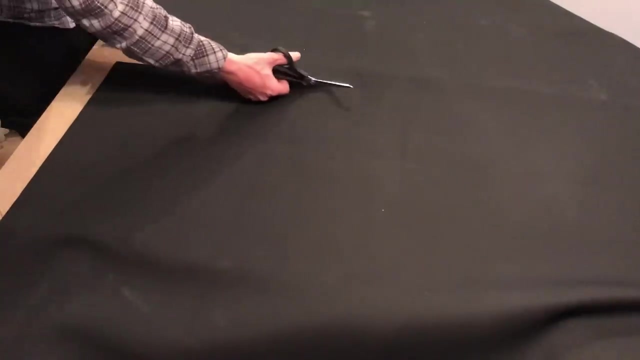 And if you do this project, don't do what I did: Actually sweep down your surface before you start cutting fabric, because I've got sawdust everywhere. It came off, but it was a bit of an unnecessary pain. So the next bit is going to be potentially a little bit tricky. 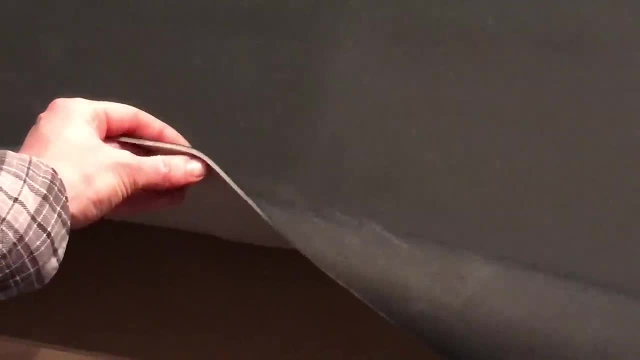 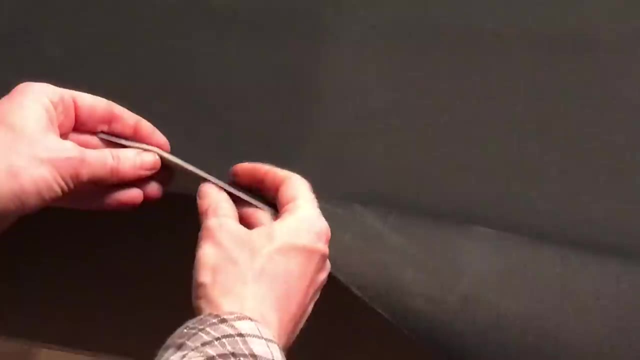 This is actually sort of like an expanded foam on this side. So if you stretch it too much then it's going to put tension and make it feel really thin and potentially a bit cheap. So I'm going to put contact adhesive on the board. 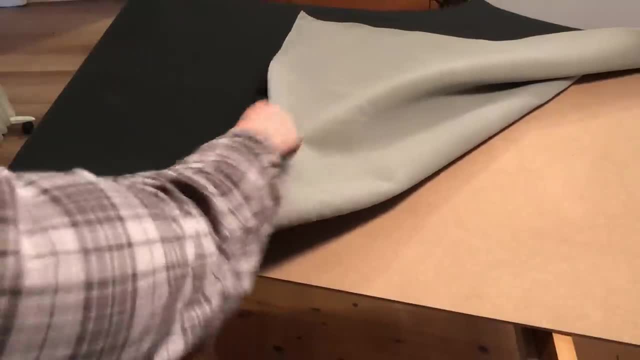 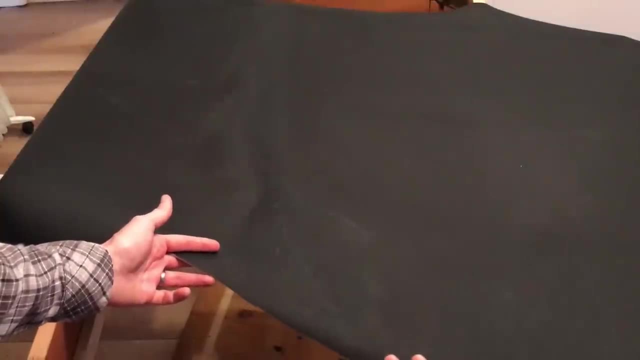 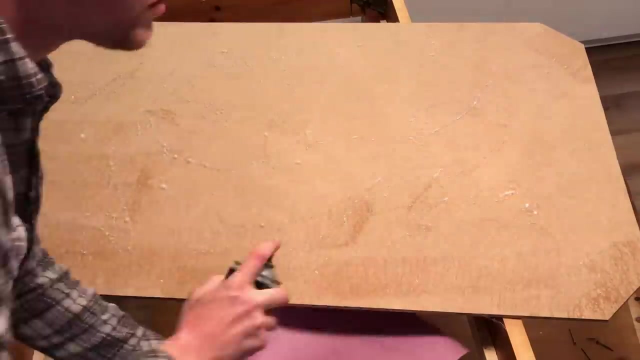 Lay it over, Hopefully do it straight, Flip it over and then just tension it a little bit and hopefully put some staples in. Wish me luck. And as it turned out that Nemesis spray glue was better than I could ever imagine, It's quite a weird texture. 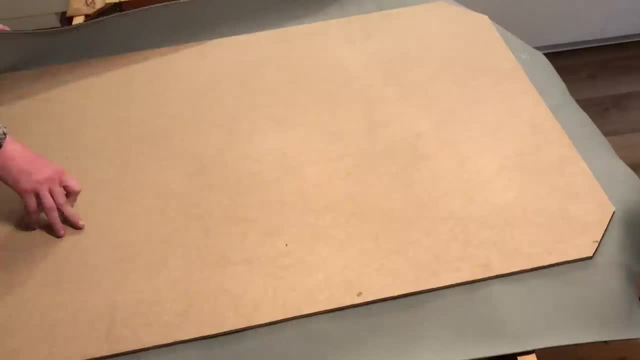 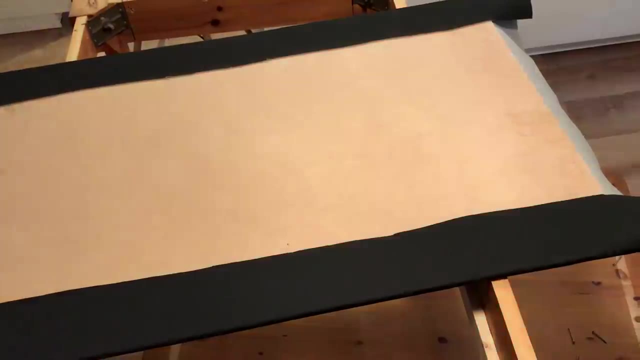 It sort of comes out like the Spider-Man webs: It's really stringy and just sets almost immediately on touching but still gives a little bit of rework. It's just fantastic stuff. So the next bit: I sort of made a bit of a meal of. 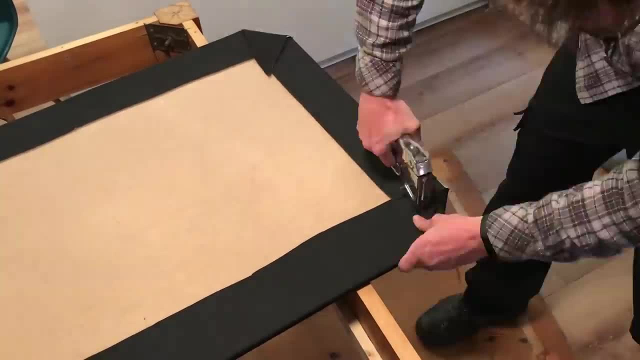 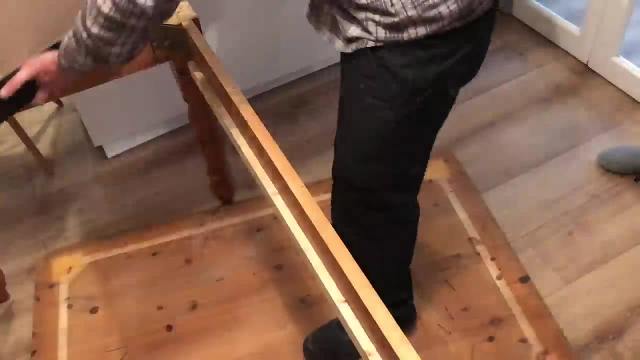 Cutting the corners and folding it in shouldn't be this difficult, But I certainly made it this difficult. What I should have done in retrospect is cut it across the diagonal and folded it in, But I staple, gunned it and it's just worked out fine. 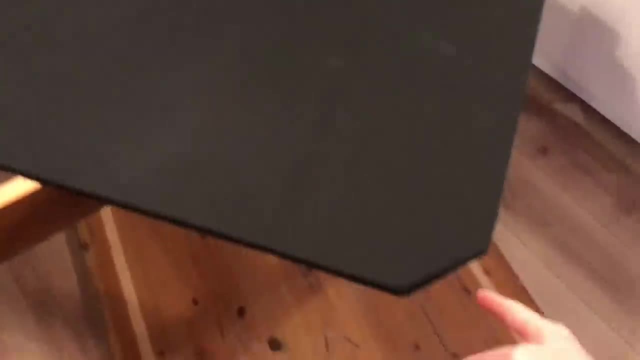 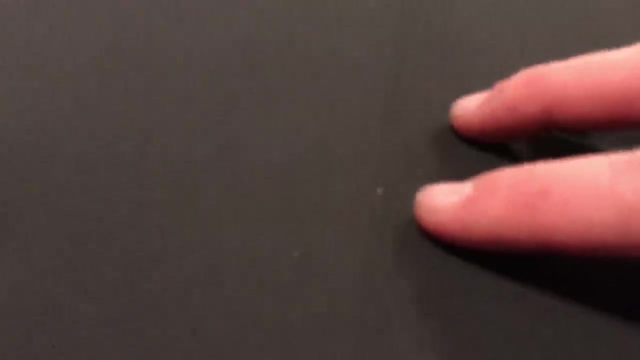 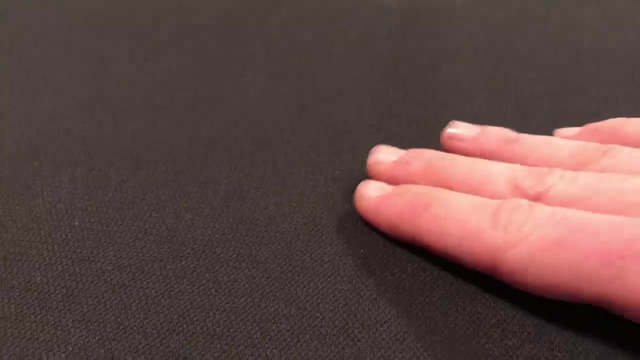 Okay, despite an absolute horror show on these corner sections, it actually looks and feels pretty good. It's got that- I don't know if I can capture this- that nice soft feel there, which is what I was looking for, And it actually looks pretty neat, to be quite honest with you. 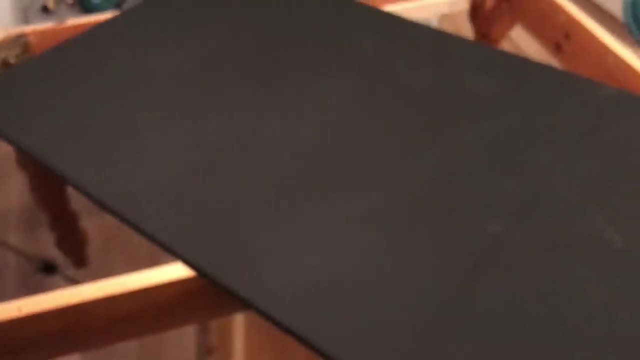 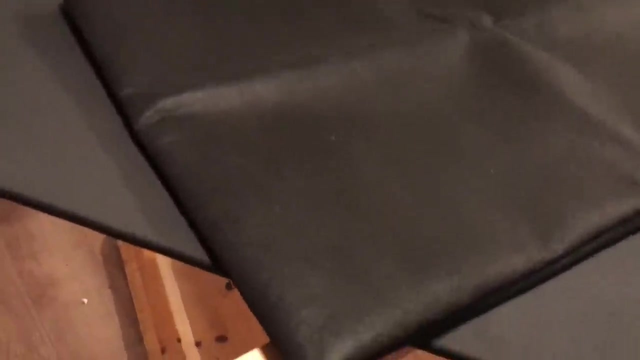 It does almost raise the question: Is it worth it? Is it worth covering it in felt? Well, you know, after all, that I've got the felt out and it sort of has this weird sheen to it. You know, I'm not convinced by that at all. 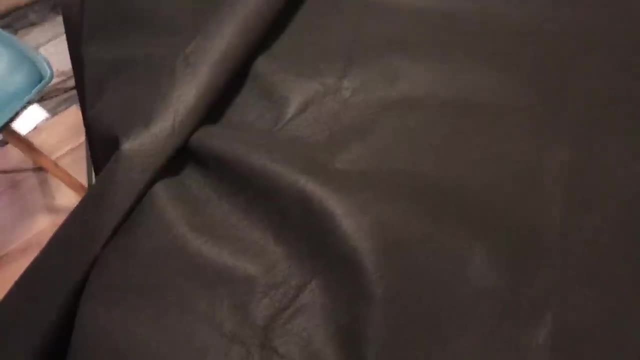 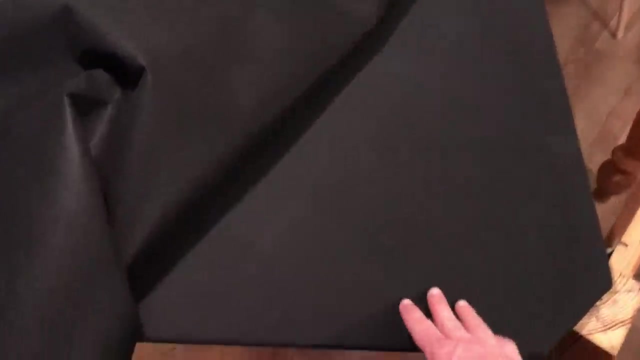 Do let me know in the comments what you think. but it sort of looks like a bin bag, you know, And maybe just go with this. It looks cool and it feels great. It does feel a little thinner, though. That's the only downside. 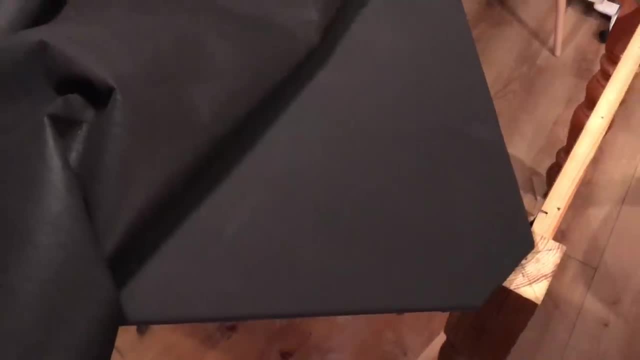 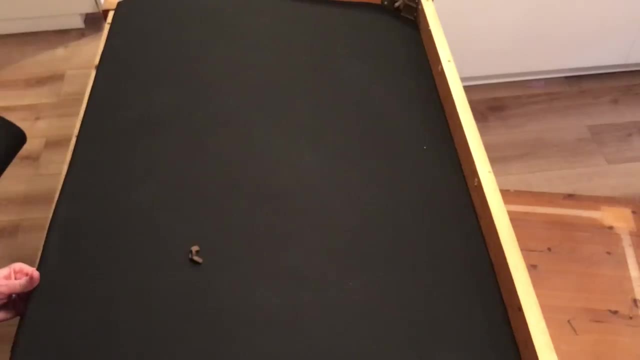 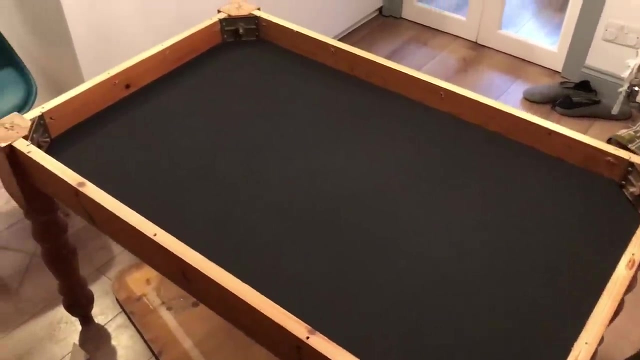 I suppose I could do a double layer in future. I'm going to get it assembled and, yeah, roll a few dice, see what it looks like. Well, I don't know about you, but I'm pretty happy with that. How much was spent on this, which is next to nothing. 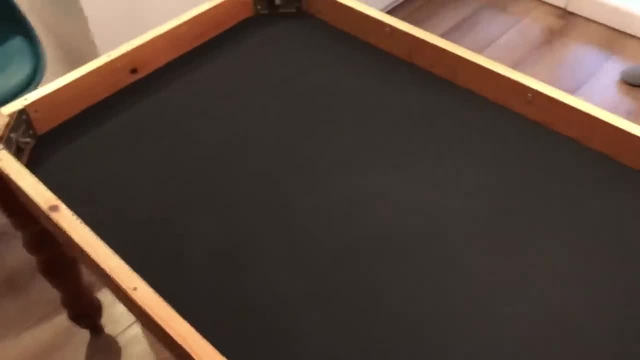 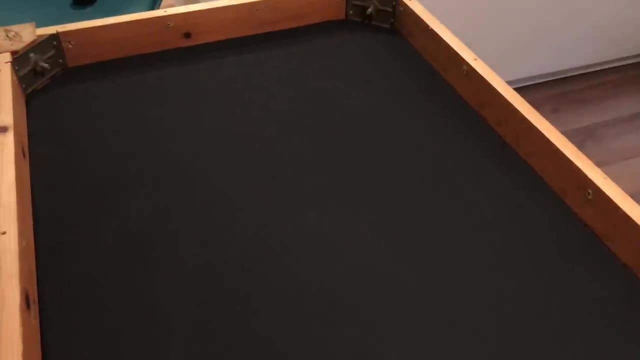 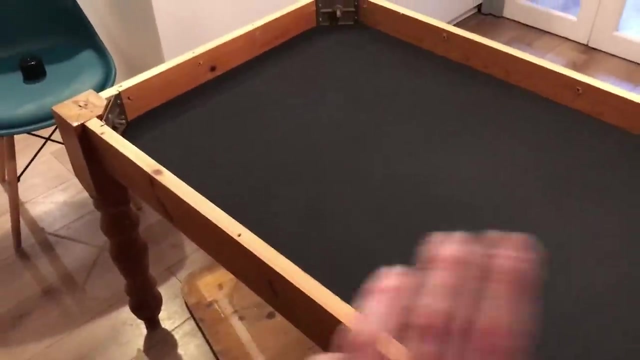 That is a really cool surface. I'm going to set the camera up, roll some dice so you can get a feel for what the components look and sound like on the board- Fantastic. Obviously, there's more to be done on this project. I need to find a secure way of attaching and reattaching the tabletop. 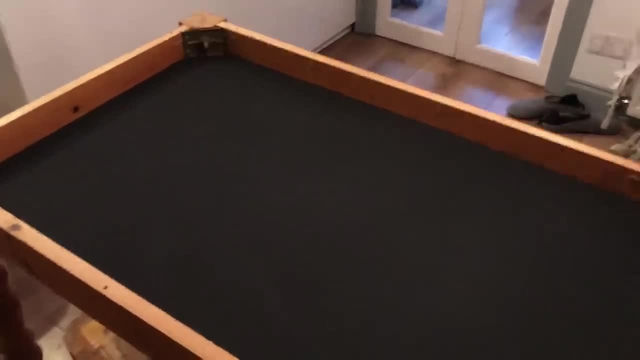 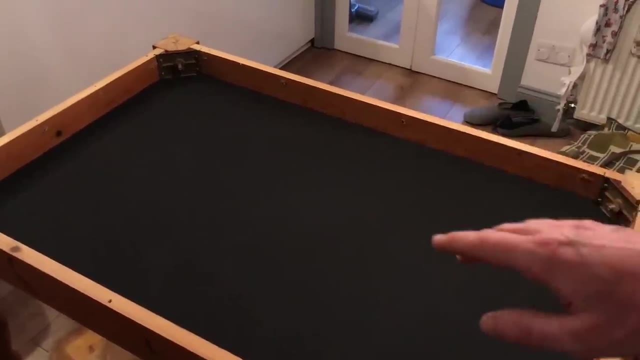 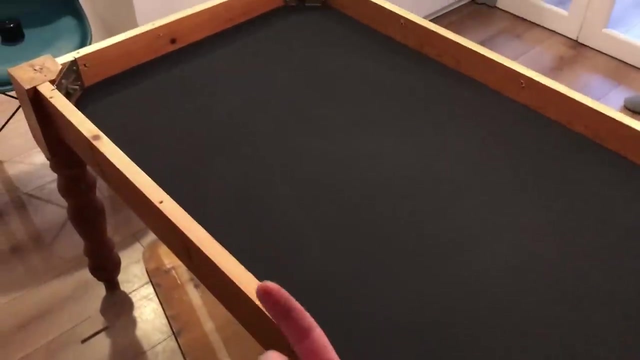 I was going to put some gas struts on so I can have the table folded at the back, because I mostly play solo and co-op games. So just having three side access is going to be perfectly fine. But I think in the initial case maybe what I'm going to have to do is put some little door locks on the underside to hold the tabletop in place. 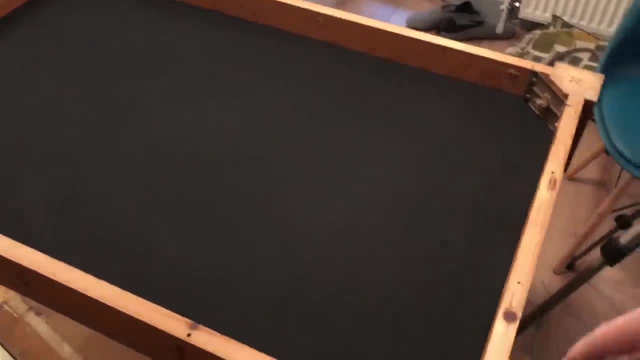 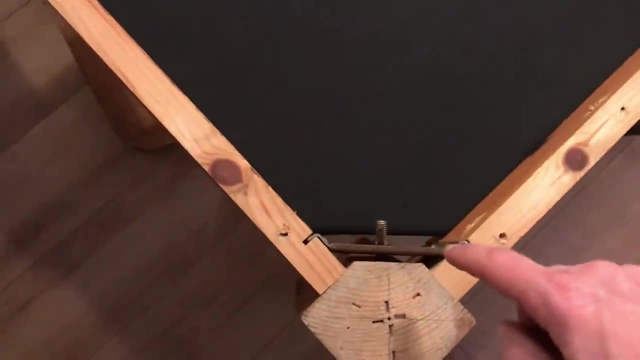 So it doesn't slide around when not in use. Alternatively, I could create some dowels, but that's going to be a little harder. Obviously, there's finishing to be done Down here. there's gaps where I've cut a generous clearance. 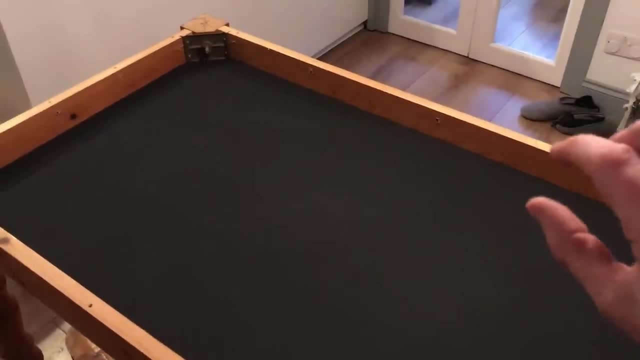 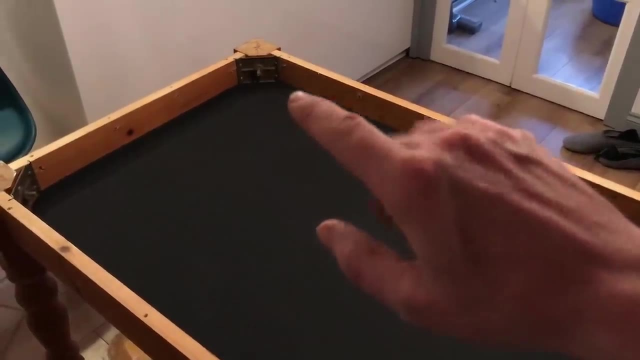 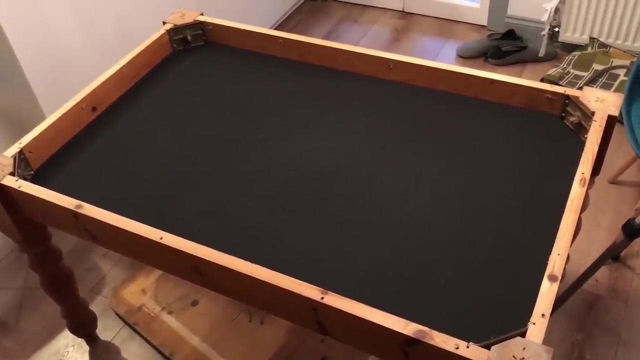 But it's my intention to board out the sides, maybe have some thicker battens covered in the same material With maybe a bit of a clever mitre block in the corners to hide that detail. But that is the gaming table. I'll leave you with some shots of some components also the tabletop on and off. 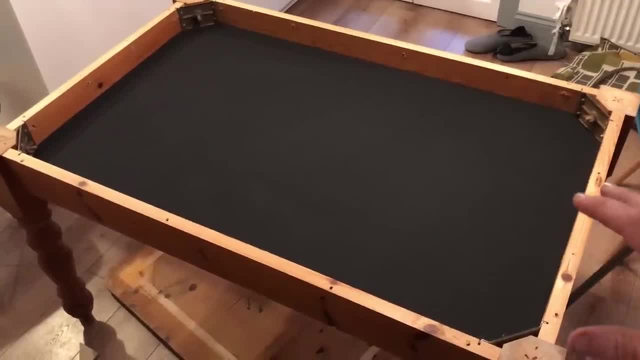 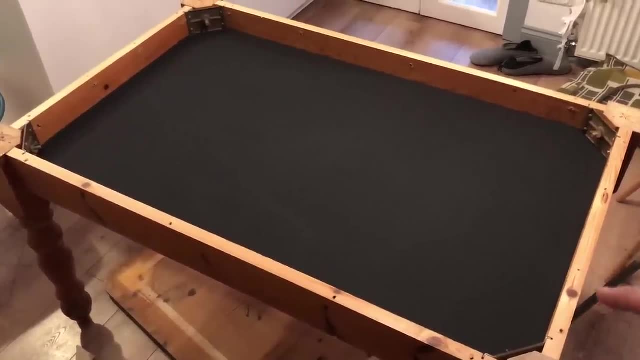 And if you like this project, do subscribe, because I'm doing a lot more on this. I'm going to be obviously putting the finishing touches and then having a bit of a review and seeing how I could have done things better. I think I'm probably going to make another one, because this table is only a charity shop find. 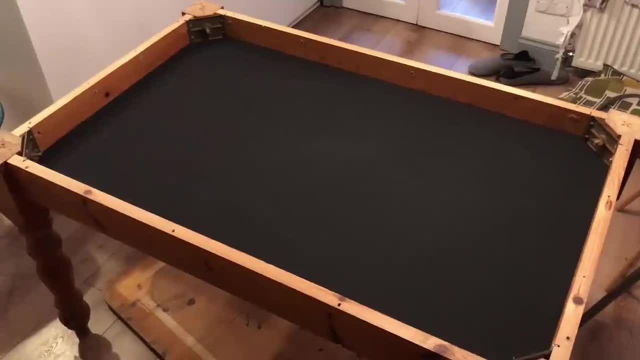 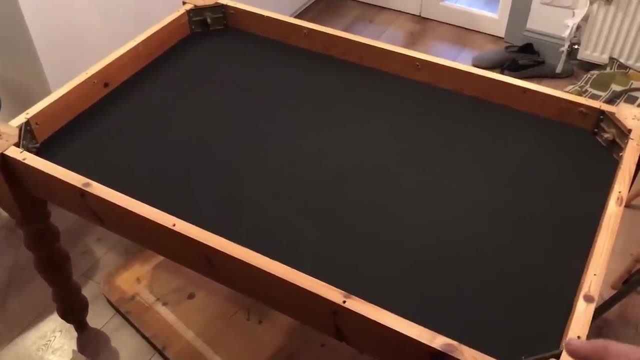 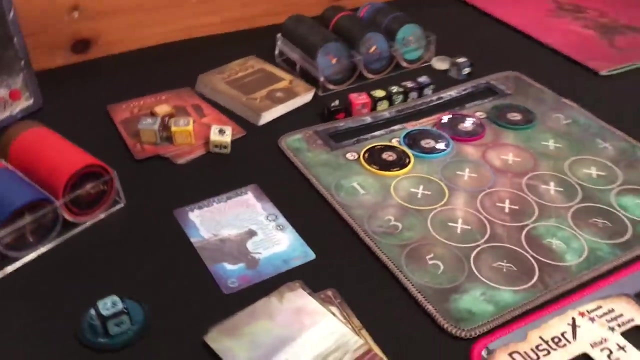 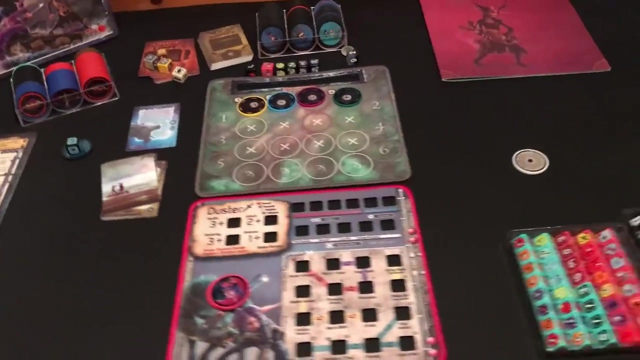 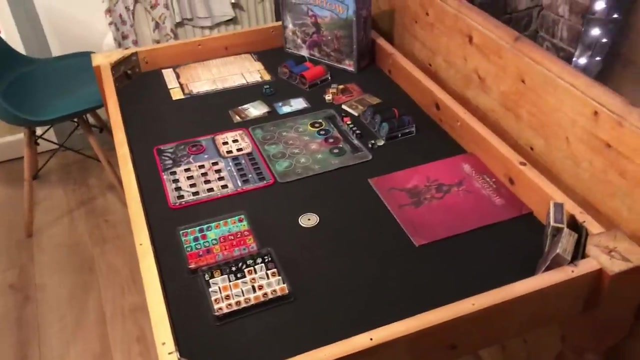 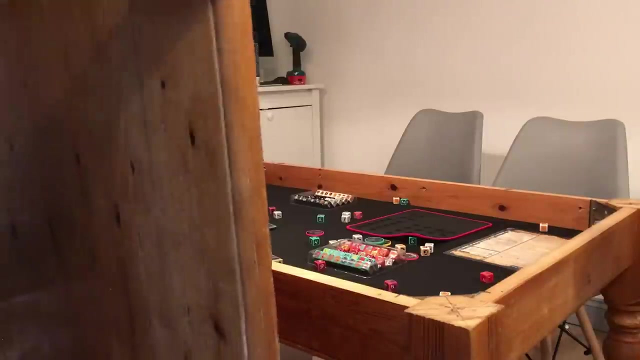 And I think you can probably make an entire gaming table for around £50,, table included. So until then, do like, subscribe and comment, And I'll leave you with some more, Some component shots. Thanks for watching. We'll see you next time.